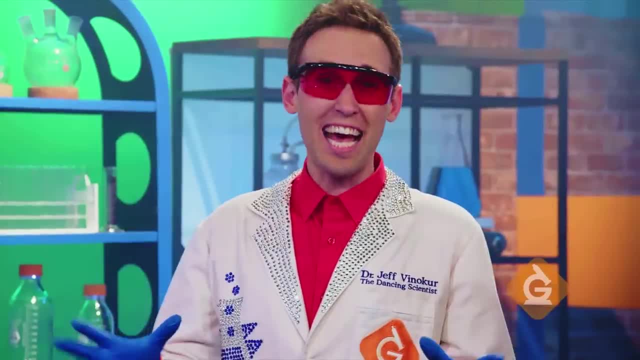 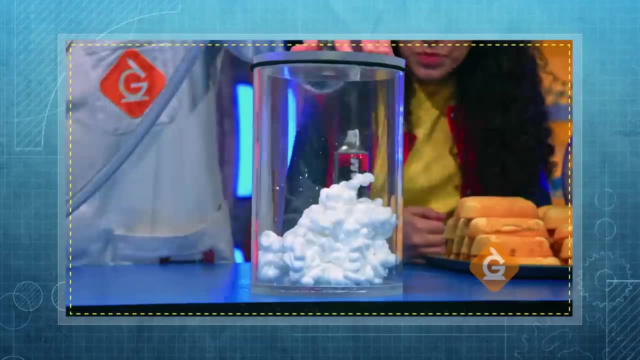 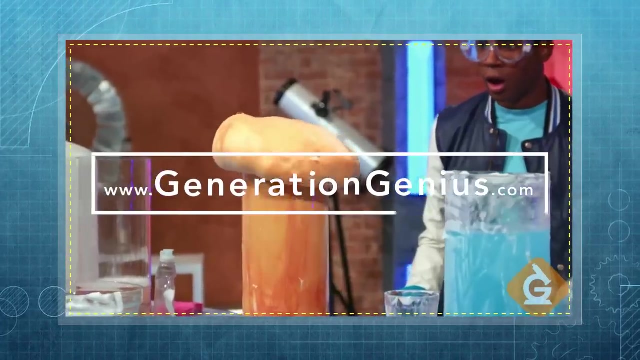 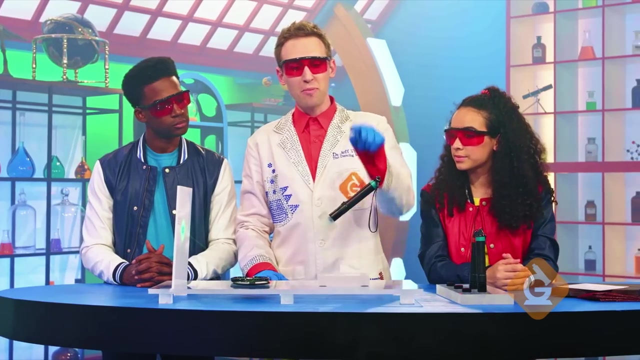 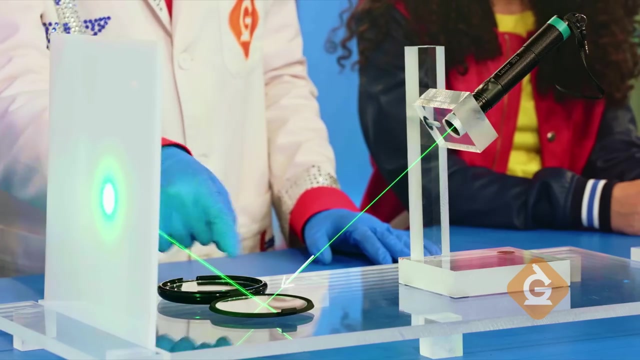 To help us understand what just happened, we need to understand light reflection. Let's break it down. This is a model of light reflection made from a light source, a reflecting surface and a viewing screen. The laser light is bouncing off the mirror, making a V shape. 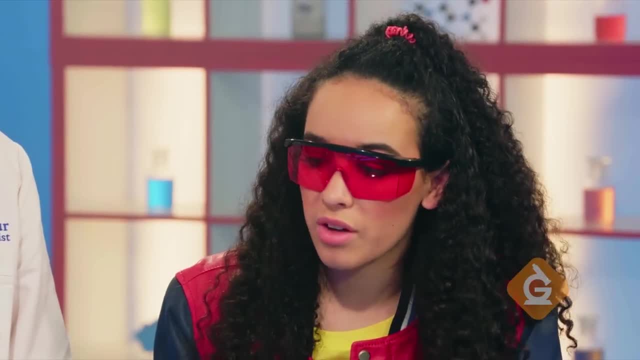 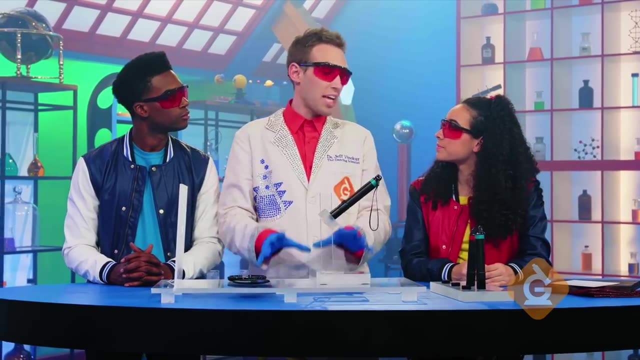 This model allows us to test how light will reflect off other objects. Everyone knows that mirrors are good reflectors: They're shiny, True, but non-shiny things reflect light too. Let's test some different materials using our model. Look at this. 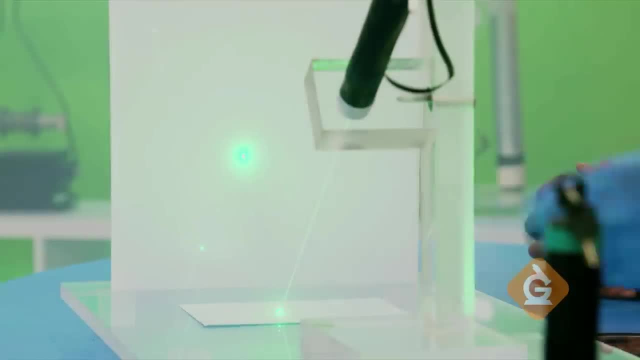 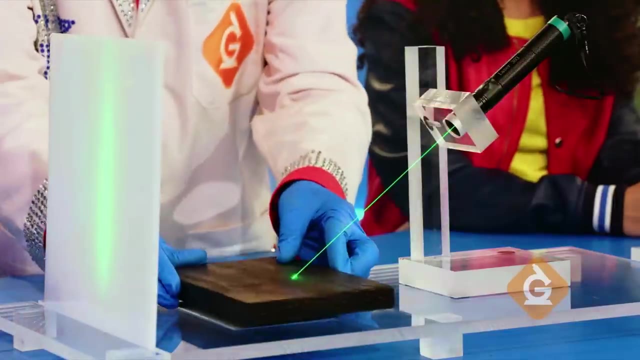 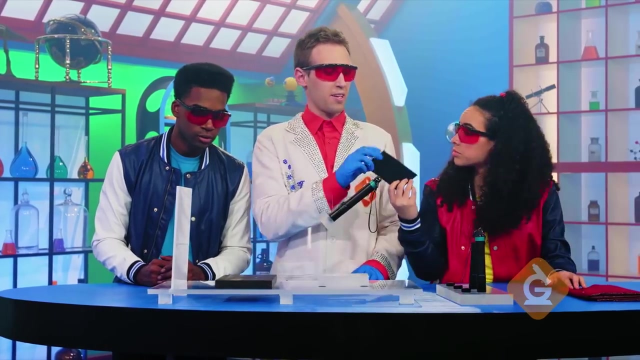 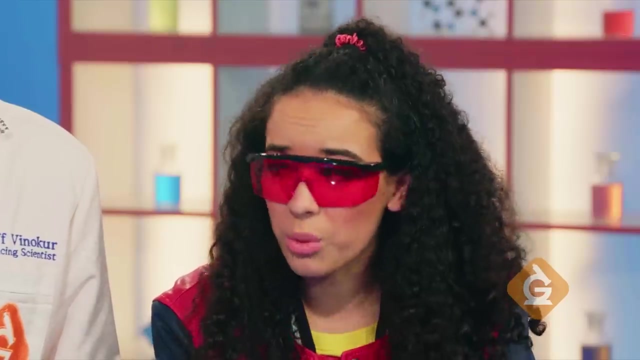 Piece of white paper. White paper is a good reflector too. Dark piece of wood. Dark piece of wood isn't as good, but still reflects a little bit. Black cardboard- That's strange. I thought black objects don't reflect any light. 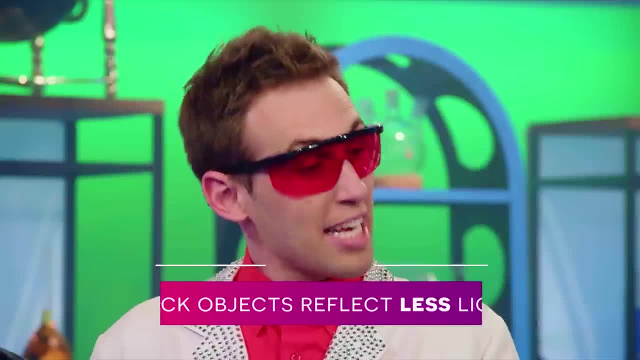 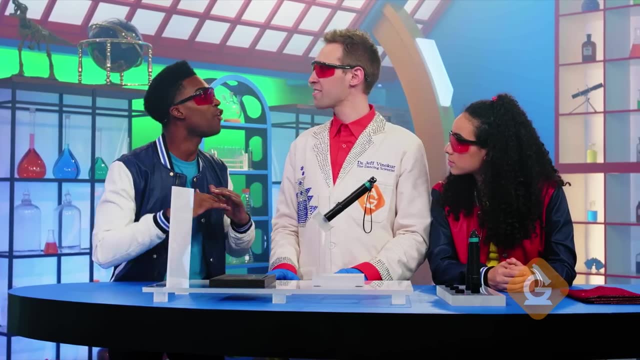 Black objects reflect a lot less light than white objects, but they still reflect light. I get it. If an object didn't reflect any light, we wouldn't be able to see it, Like if we turned off all the lights. I'm on that. 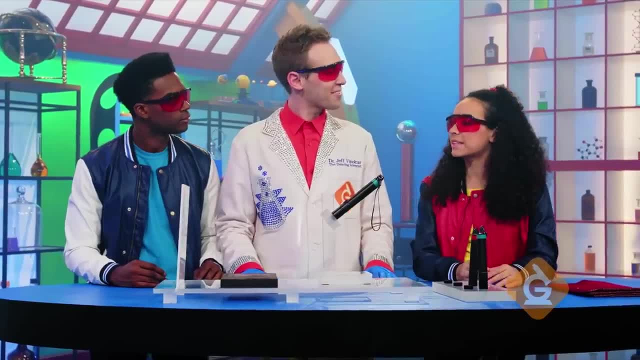 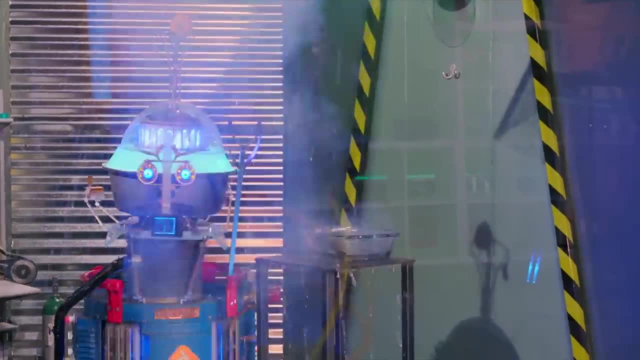 Sorry, Without a source of light, we can't see anything, because our eyes don't produce a light. But what if they did? Hey kids, If you want to watch this whole episode and more, tell your teacher to sign up at GenerationGeniuscom. 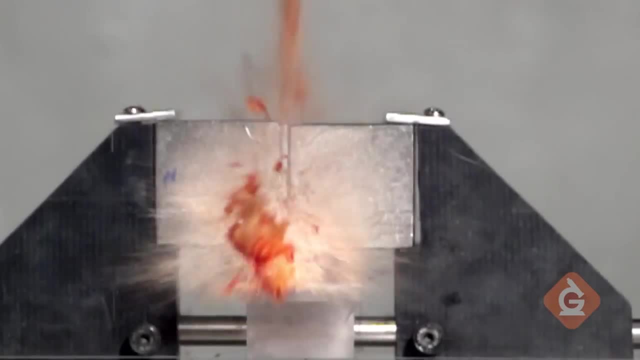 We cover all science topics in grades three to five and you get to watch it in class, But only if you tell your teacher.